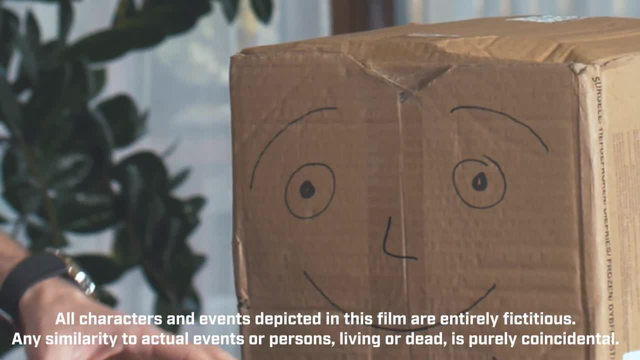 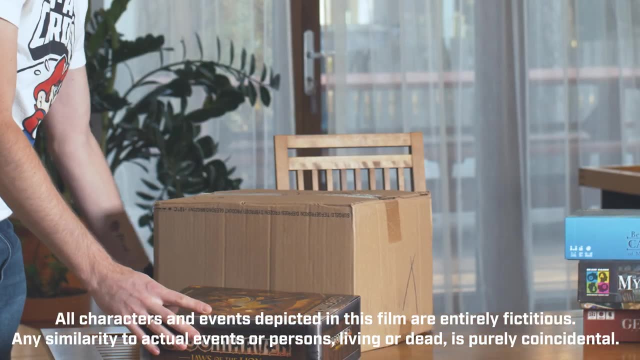 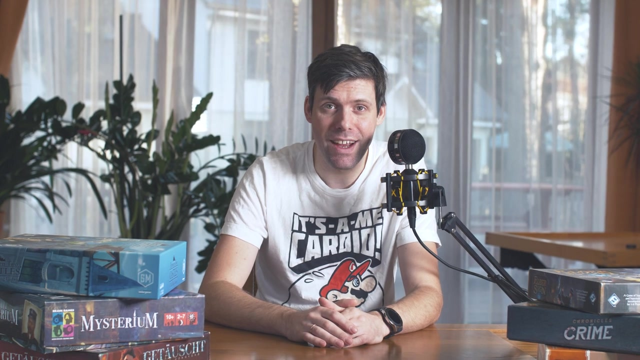 gloomhaven. it has different characters, different abilities. each player gets a new deck and you go through different scenarios and it takes an hour or more to play through each scenario and wow, that sounds like a lot of fun. tip number two: be patient. kids aren't patient by definition, and their 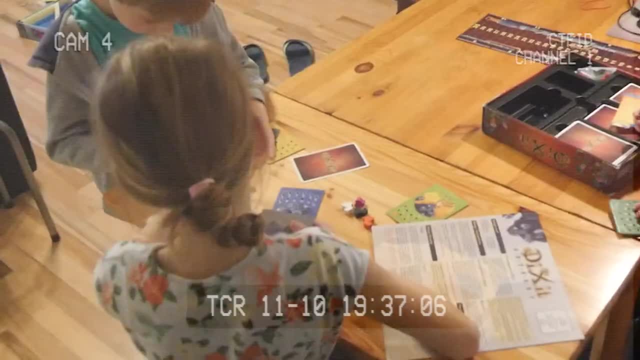 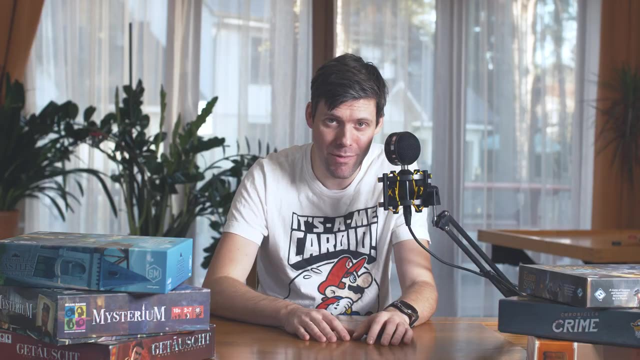 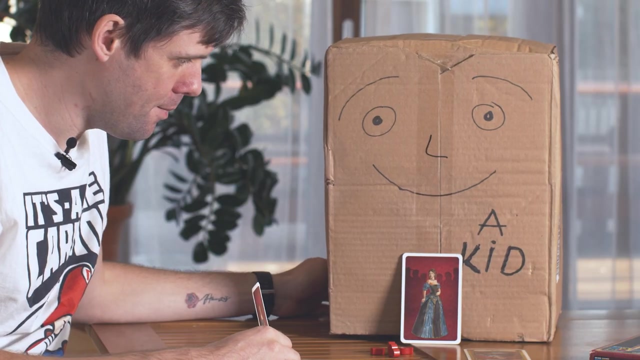 attention span is well non-existent. listen to them and let them know that you listen to them as well. and if they ask for the 35th time how far they move when they roll three, you carefully explain that it's three. hey dad, so what do i do on my turn? so you draw a card and then you play one. 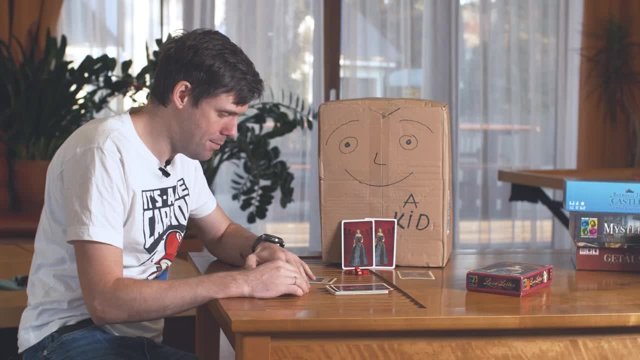 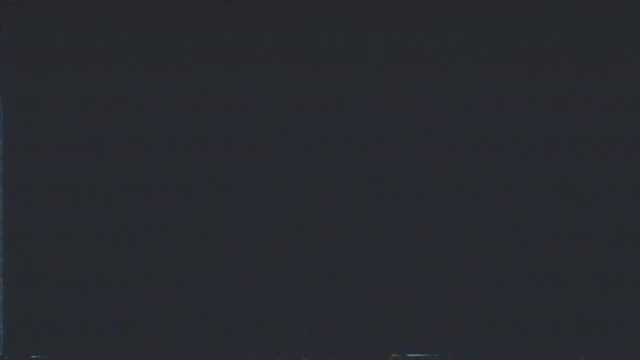 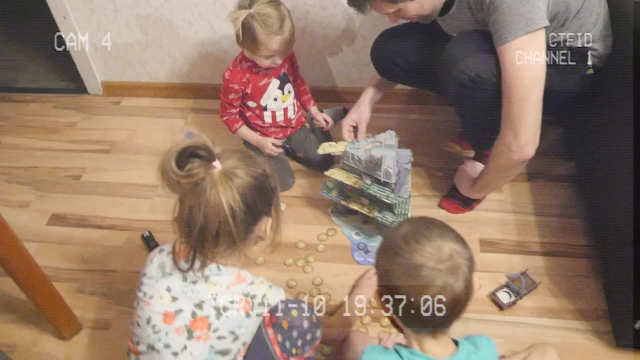 oh one, yes one. so do i play it now just play. you draw one card and play one number three. let them see you enjoying this. when i mentioned that you will have to play all those boring games at the beginning, there's another thing you have to do when you do those, let them see you enjoying this. 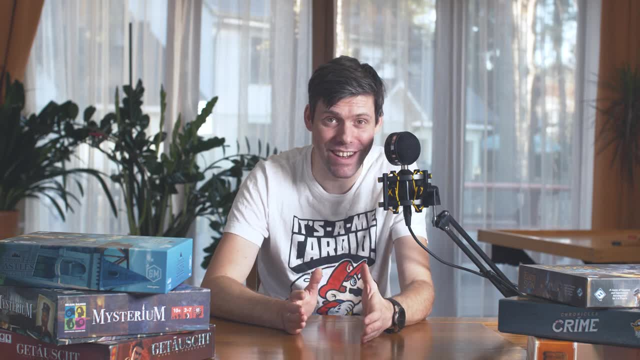 let them know that the time spent together is actually fun, because i know, as i mentioned before, you're gonna be so bored playing that lotto, but let them see that you're enjoying it. don't think about the lotto- it is. it is not a good game, but you're spending time with your kid and that is. 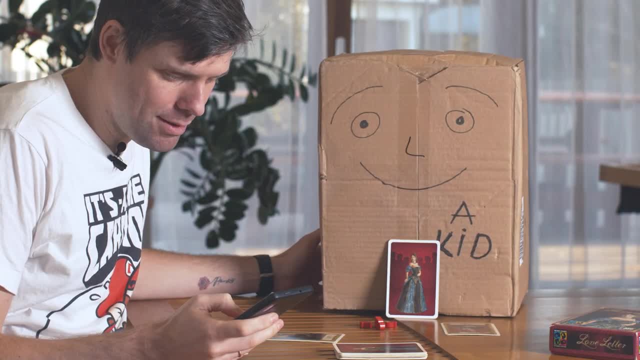 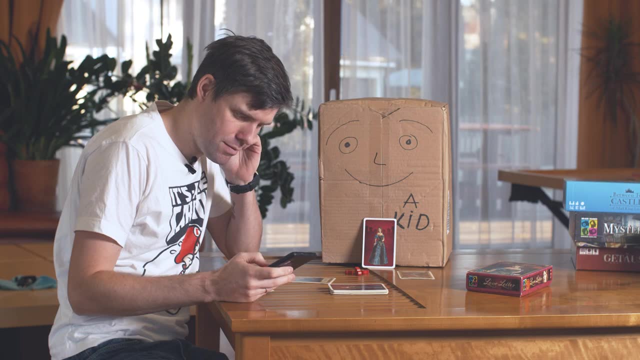 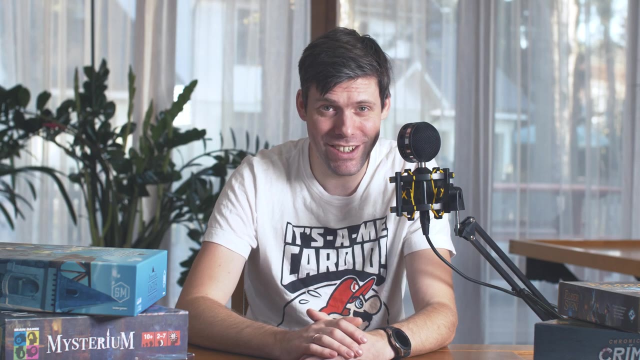 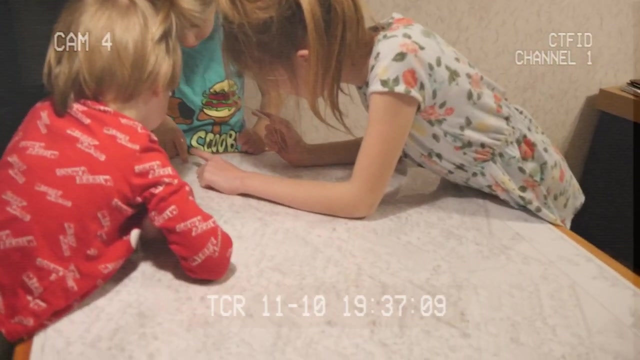 what's important. hey, dad, are you having fun playing this with me? well, oh, we're playing a game, um sure, yeah, so much fun. tip number four is: don't let them win. well, here's an important one that's gonna help them in their life, not just as a board gamer. let them win sometimes, but not all the time. i mean one of the 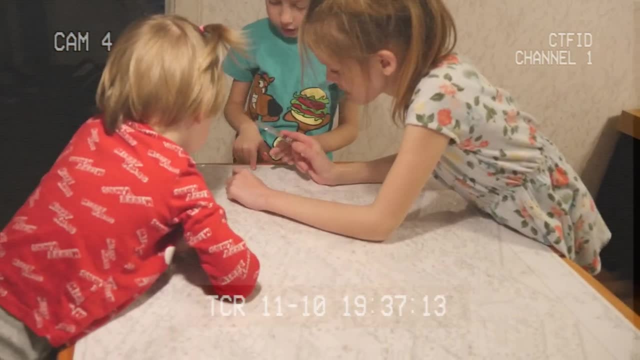 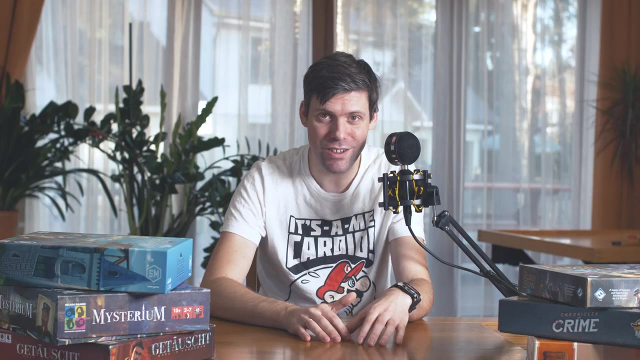 biggest skills you can learn is to lose. it's going to be very useful in life. i've seen so many 10 Like well, three-year-olds that they just lost in a small simple game because their parents had always, you know, given up to them. 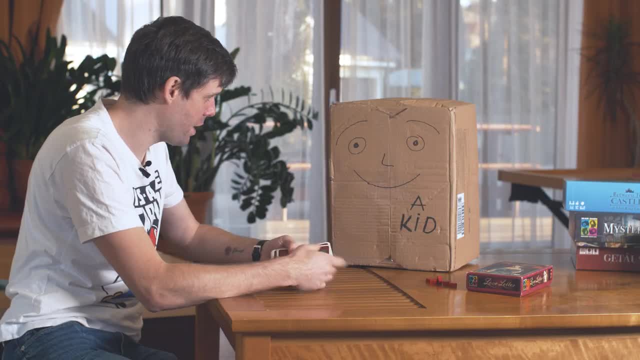 It's horrible. Don't do that to your kid. Hey son, do you want to play a game? Yeah, dad, I love playing games and winning. Cool, Let's see how you do this time. So here's a card for you. 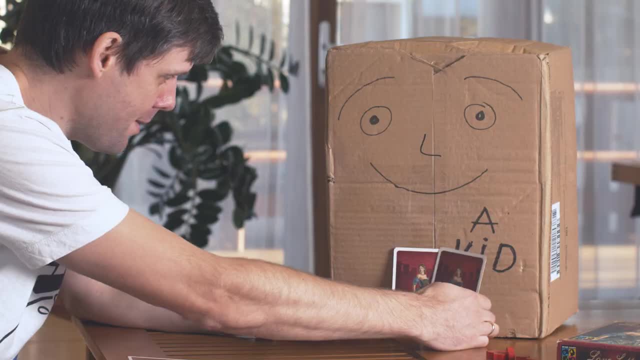 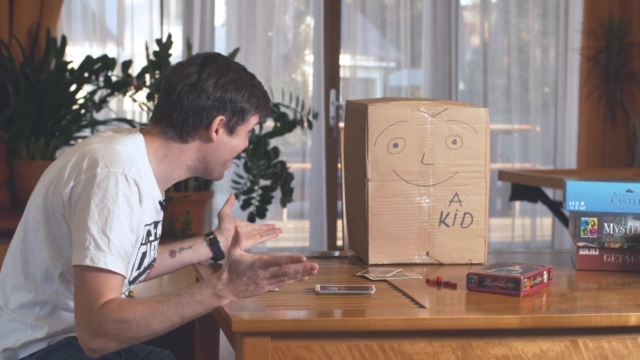 And here's a card for me. And then you get another one. Play one, I'll play this one, You win. But what if I play this one? You would have won as well. But what if we played that game? You would have won. 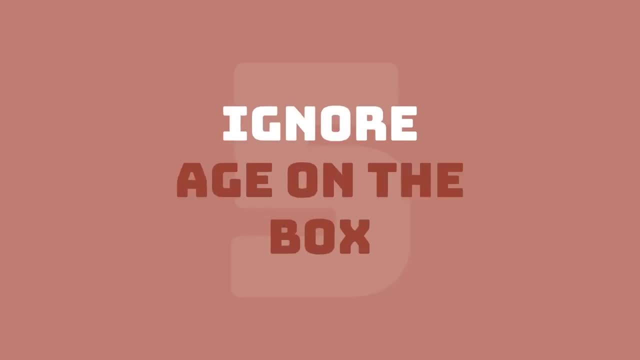 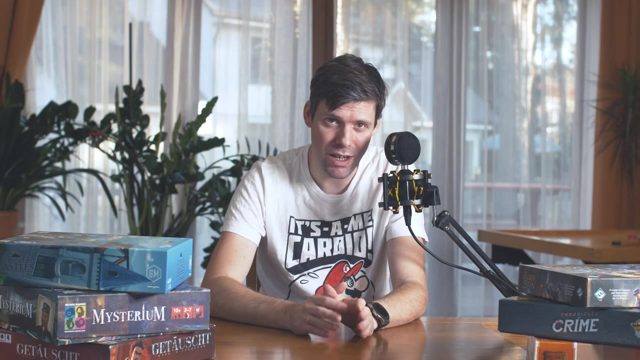 And the last tip for today, number five, is: don't look at the age on the box. I know what I said about lotto and memory games, that you should start small, But if you feel your kid is ready and you'll know it, trust me, try those bigger games. 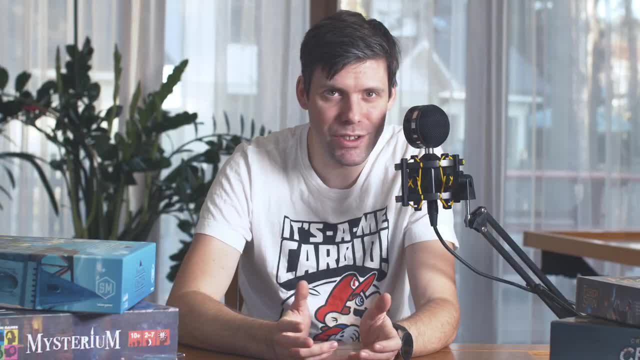 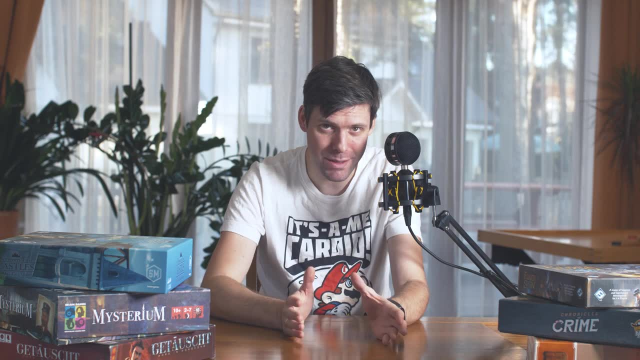 For example, if it says eight plus on the box and your kid is six plus, just try it. Maybe it will take longer for him to get things. Most likely they will. But with patience and using all the other tips I said, you're going to get through that game. 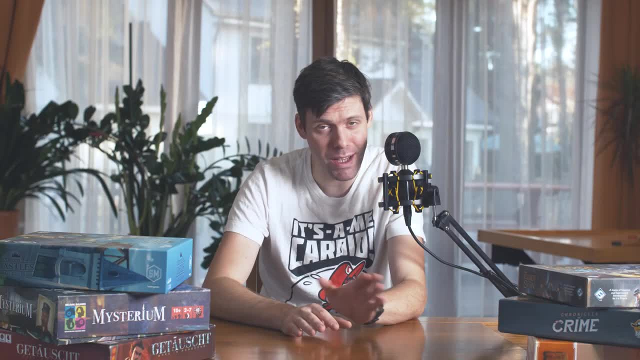 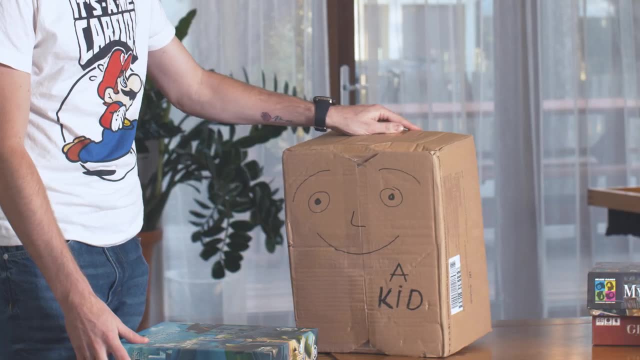 And the next time it's going to be easier and easier and easier. Sometimes it won't work, But most of the time you'll know it if he's ready. Hey daddy. Yes, son, Can we play this game? 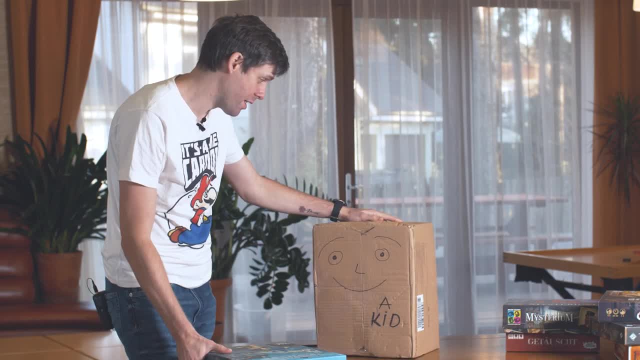 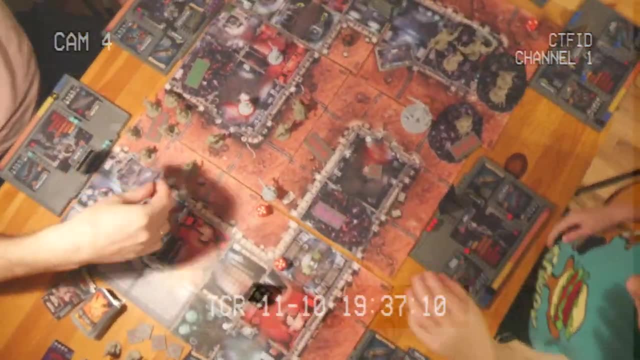 Oh no, son, It says ten and up on the box and you're only nine and a half Aw. Obviously it's not always going to work. It's just my experience and it's what helped me to play with my six-year-old Zombicide Invader. 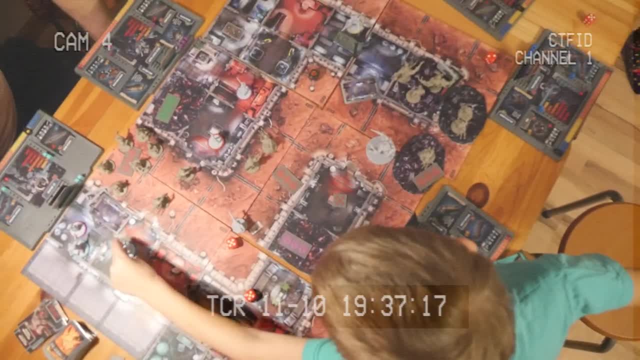 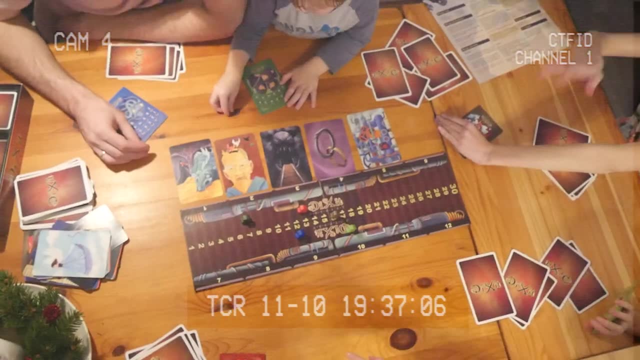 He's still struggling with it a bit, but we've been playing games since he was two years old. But I also have a daughter who's nine years old and she just doesn't like those games at all. Her cup of tea is Dixit and Just One and all these party games. 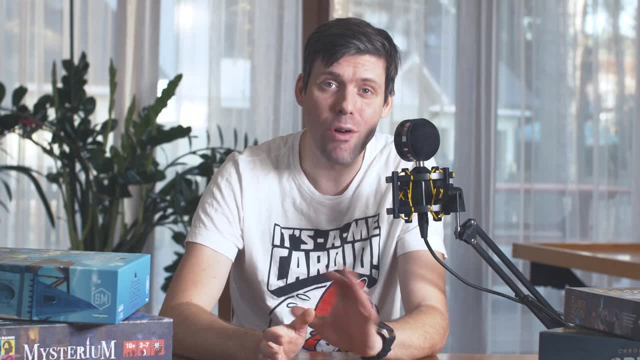 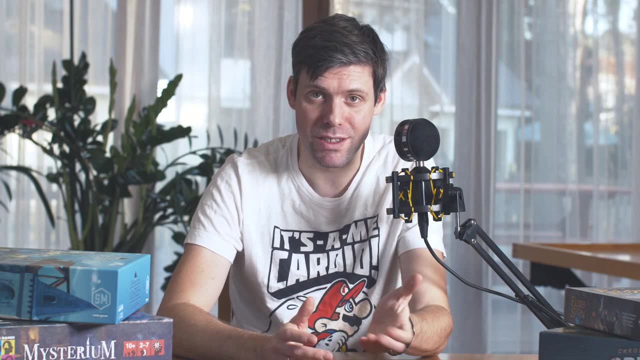 And she's never going to get into these heavy games, So it's not always going to work, but it's definitely going to help you. So try it and let us know in the comments if it did work, or maybe you're using some other things that I haven't spoken about here. 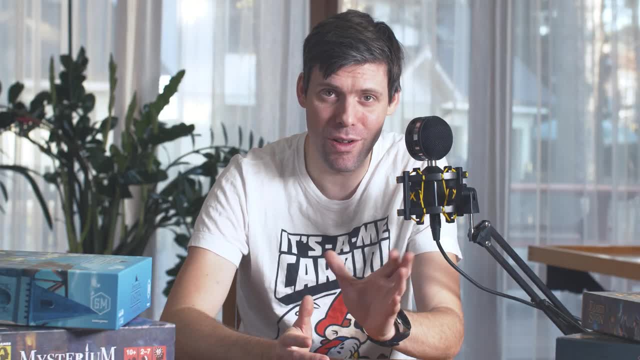 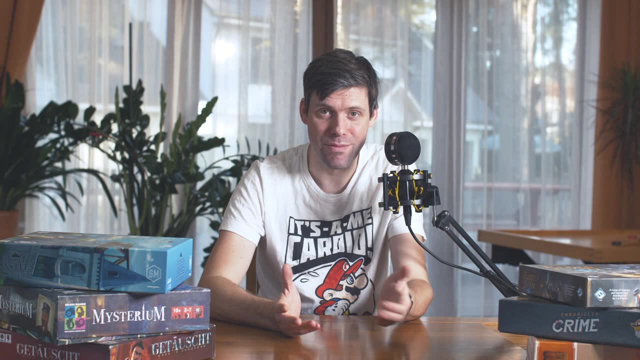 Good luck playing games with your kids. And just a small reminder: Kids usually play games to spend time, Time with you. Not especially those games matter, So you know. take that into account. But thank you for watching. Please subscribe and see you next time on Board Game Hangover. Humans are weird. 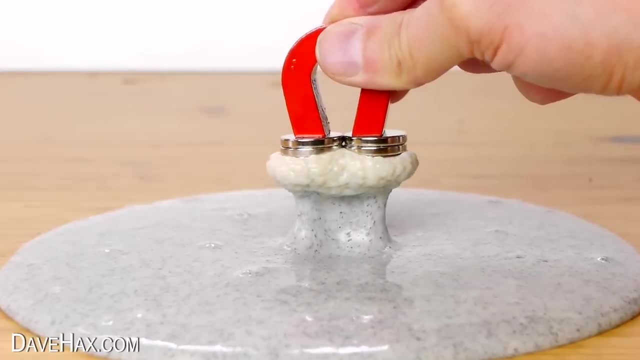 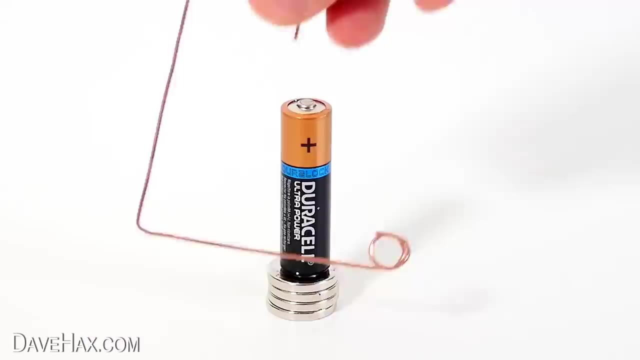 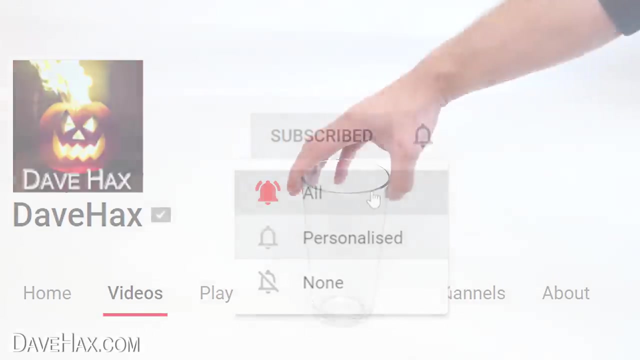 Today I've put together a compilation of some of my favourite science experiment videos which I've made over the years. If you enjoy this video, you can make sure you don't miss any of my future content by subscribing to my channel, clicking the notification bell and selecting all.